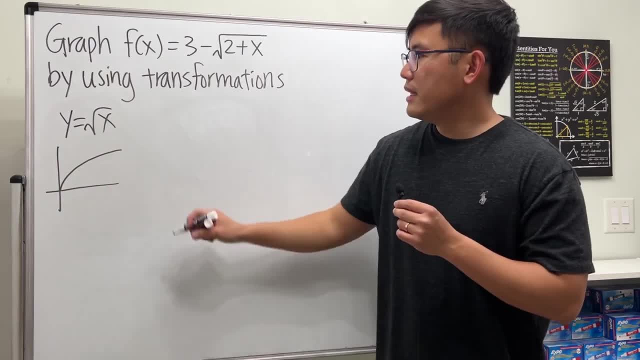 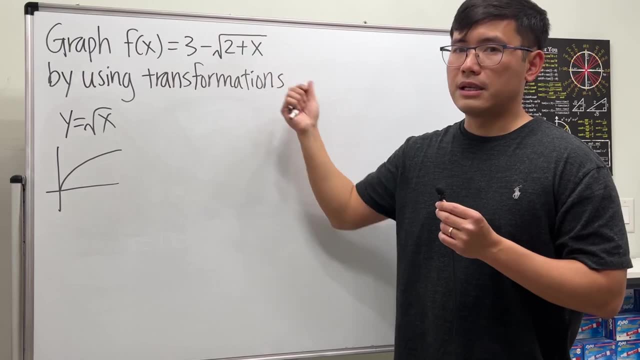 Just like a sideways parabola without the bottom half. Now let's look at this part: square root of 2 plus x, And this is really the same as square root of x plus 2.. The water of addition doesn't matter. 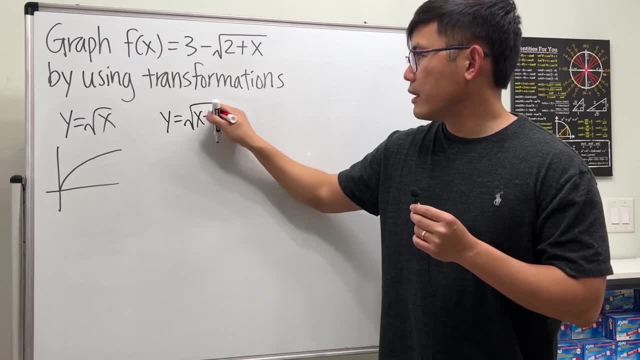 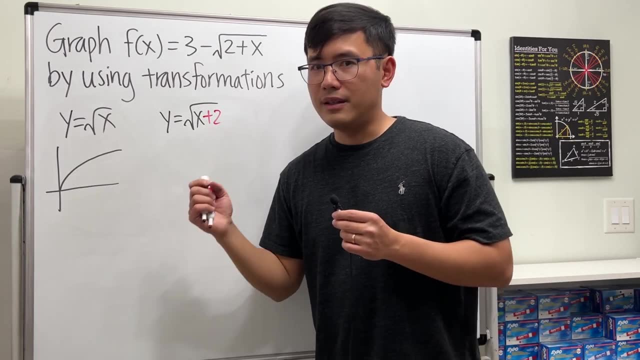 So we can just look at this part. And now, when we are adding 2 directly to the x, what does that do to the graph? And the answer is: you shift the graph 2 units to the left. It's the opposite. 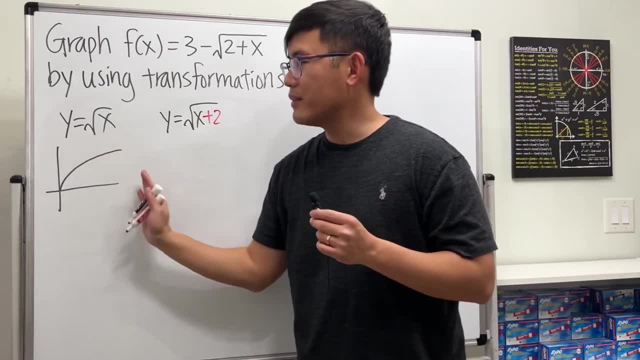 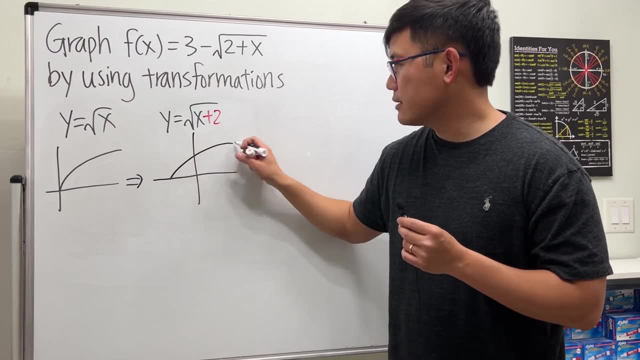 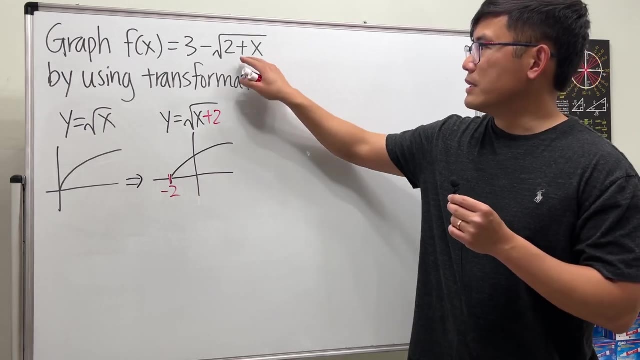 When you are adding 2 directly to the x, you take the graph 2 units left, So The picture will become right here, Starting at negative 2.. Like this: Okay, Then we see that next we are going to get this negative. 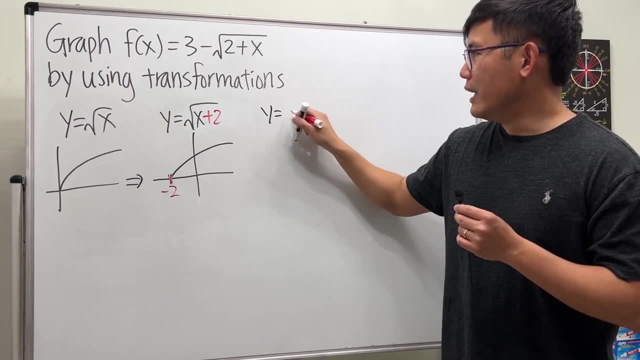 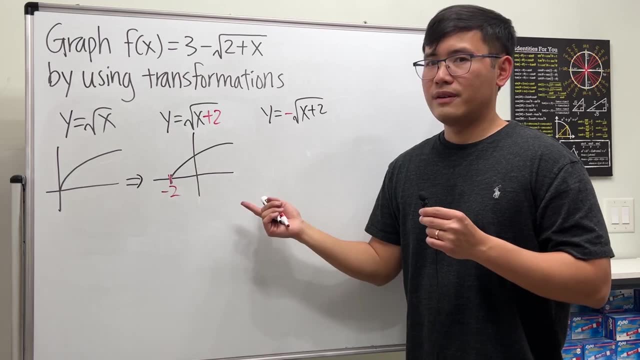 So, if you just look at this part, y is equal to negative square root of x plus 2.. What does this negative do to the previous graph? Well, it's a negative square root. Right, It's the negation of the. 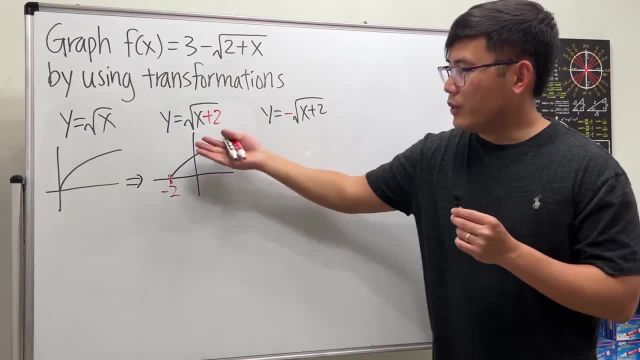 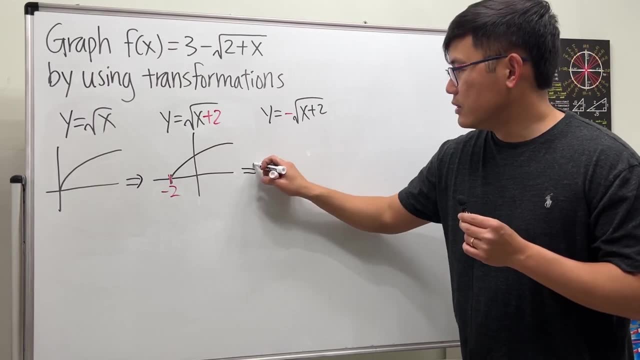 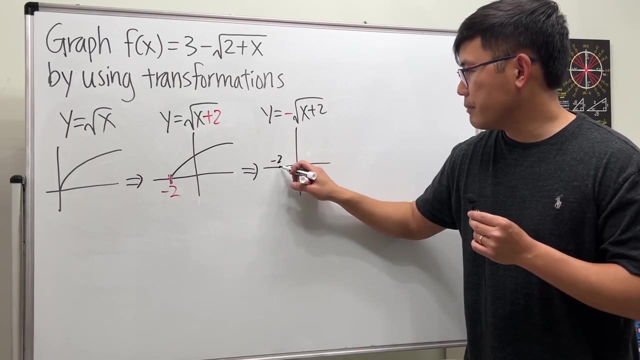 Entire equation right here. That means we flip this graph upside down. We flip this graph about the x-axis, So Our starting is still at negative 2.. That's okay, Negative 2 here, But the picture will look like this now: 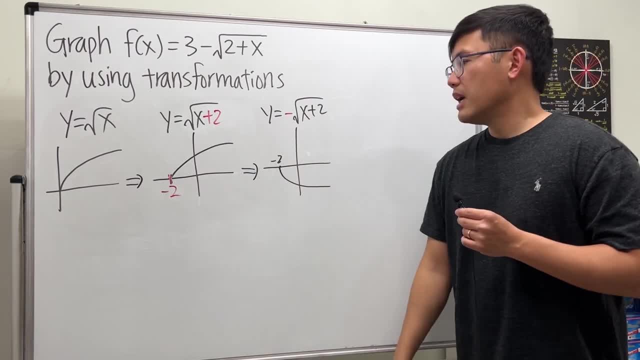 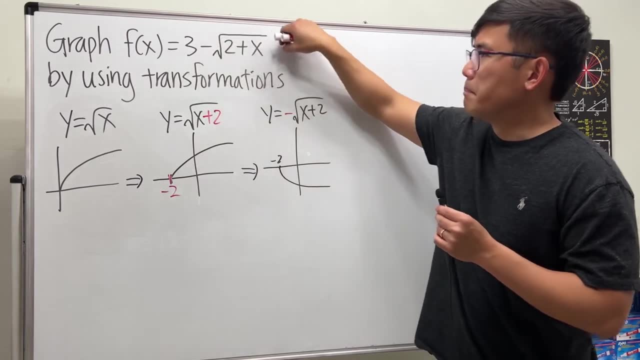 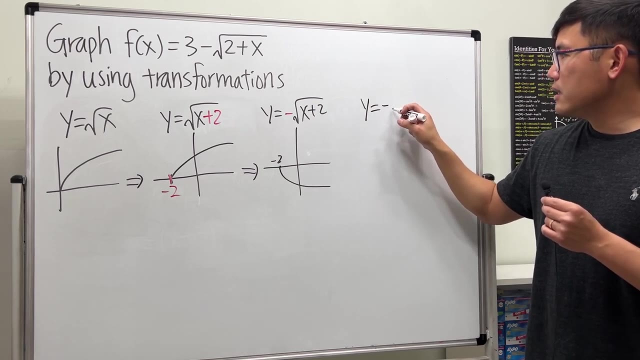 It becomes the bottom part With that negative. Okay, Lastly, we have this 3 right here, So This 3 is positive. So it's really the same as this thing Plus 3 at the end, Right, So we can also look at that as y is equal to negative square root of x plus 2 and then plus 3.. 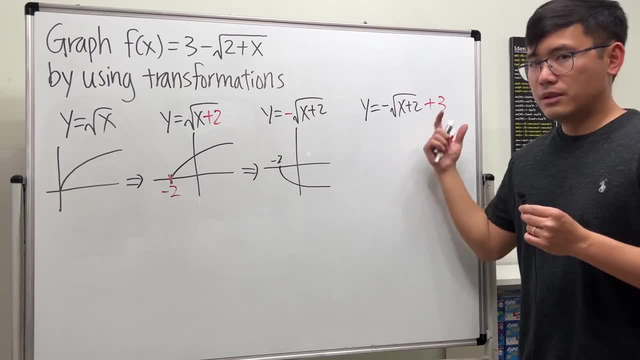 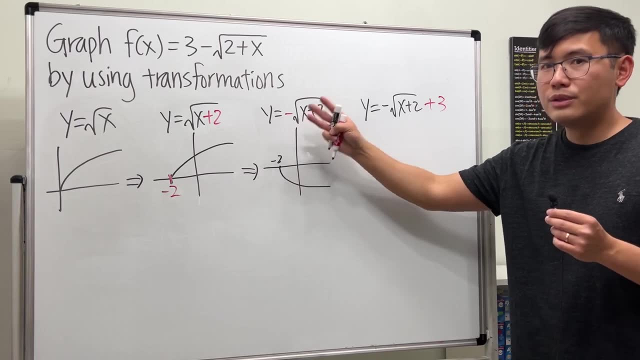 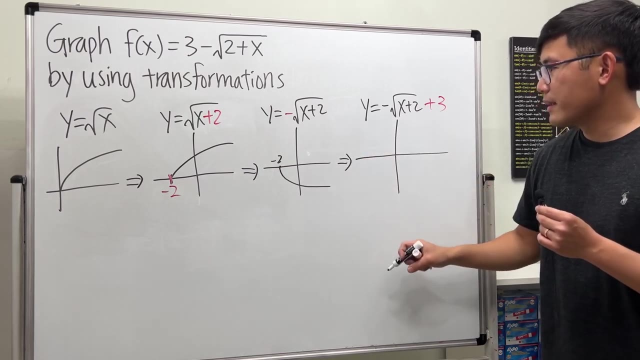 This is outside of this part. So this plus 3 tells us to take the graph right here. Go up 3 units, Yes. So here is the final picture Right here. This is my little arrow, So. So originally it was right here: negative 2.. 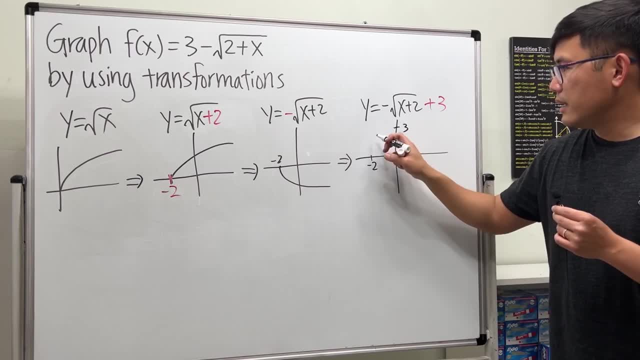 But now it's going to go up 3 right here, Right, And then we will just have a picture that goes like this: Yeah, Something like that. So It's like this. right here, I did my best. It's like that.